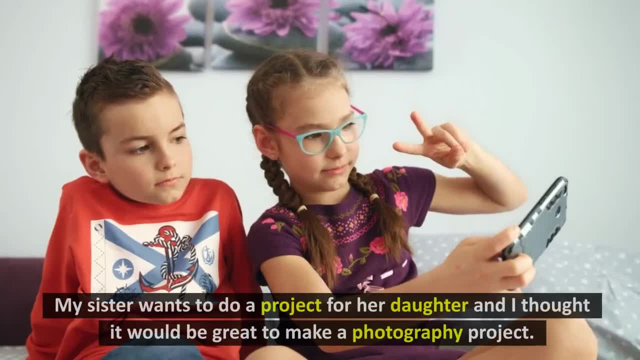 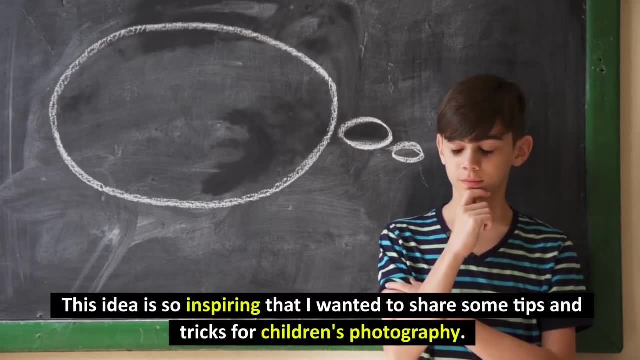 How to teach your kids photography. My sister wants to do a project for her daughter and I thought it would be great to make a photography project. This idea is so inspiring that I wanted to share some tips and tricks for children's photography. Get your child started with. 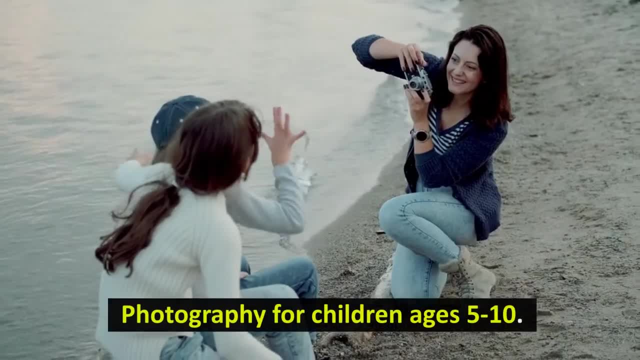 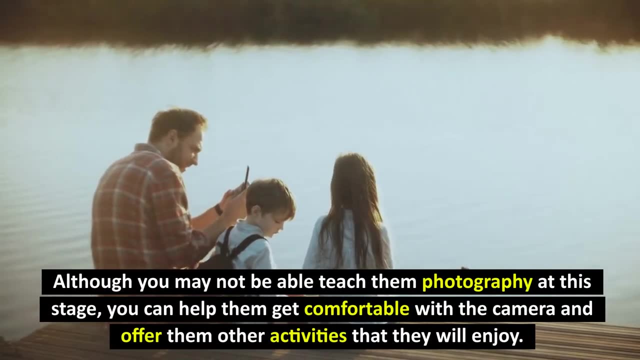 photography by doing what you can: Photography for children ages 5 to 10.. Although you may not be able to teach them photography at this stage, you can help them get comfortable with the camera and offer them other activities that they will enjoy. Teach them how to hold the camera, How do? 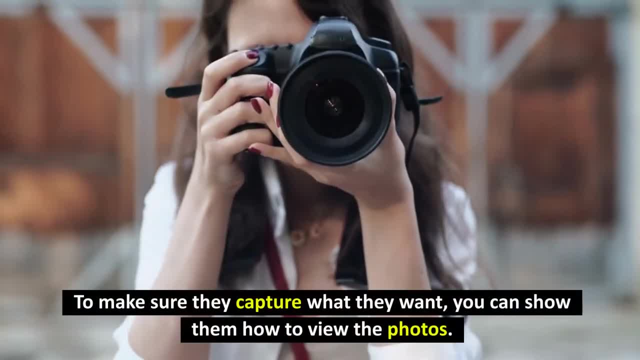 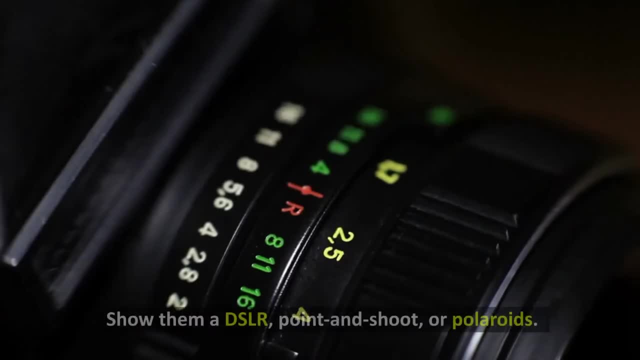 you use the shutter button To make sure they capture what they want. you can show them how to view the photos. This age group can also understand the differences between different cameras. Show them a DSLR, point and shoot or Polaroids. Don't forget to show them your cell. 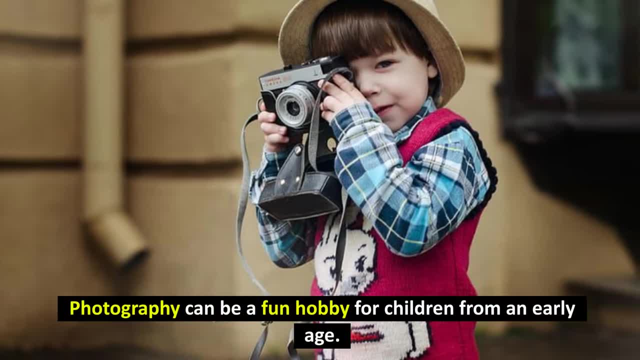 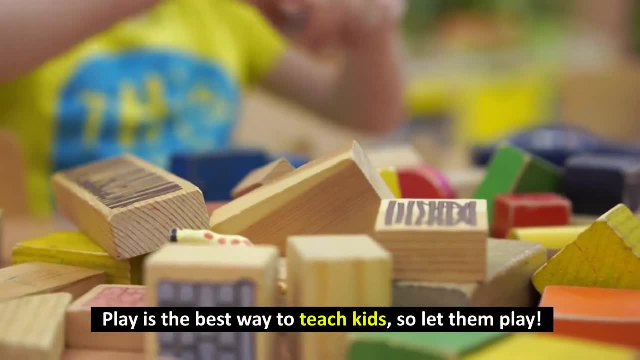 phone camera. Photography can be a fun hobby for children from an early age. This skill can be a hobby that grows over time. Play is the best way to teach kids, so let them play. Ideas for children's photography, ages 5 to 10.. 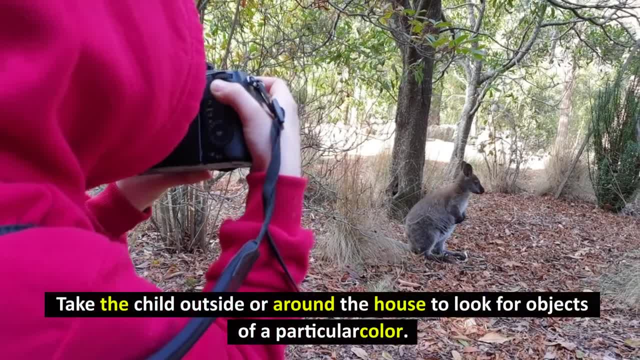 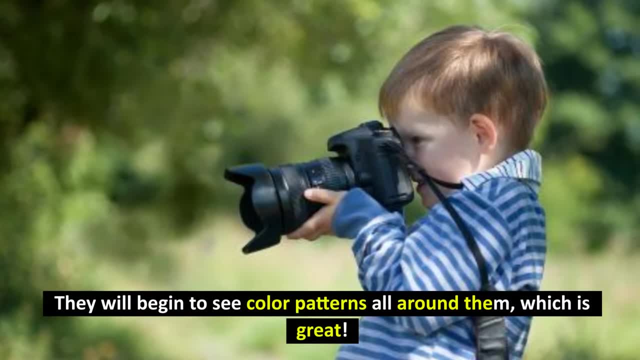 Learn about their colors. Take the child outside or around the house to look for objects of a particular color. Have them take photos. They will begin to see color patterns all around them, which is great. Ask them to identify objects starting with a particular letter, and take. 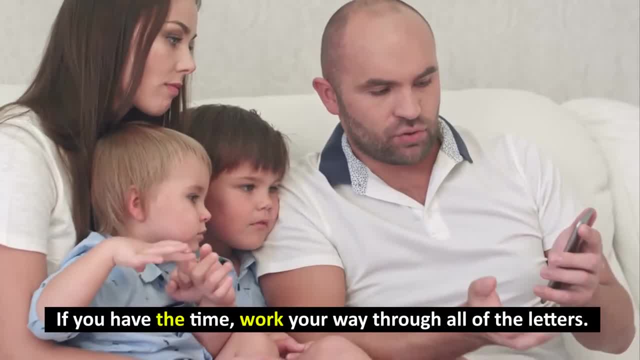 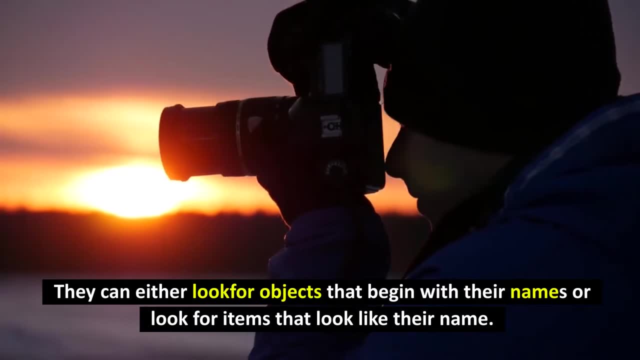 photos. If you have the time, work your way through all of the letters, Their names. They can either look for objects that begin with their names or look for items that look like their name. You can take it to the next level and create their name, then print it out. 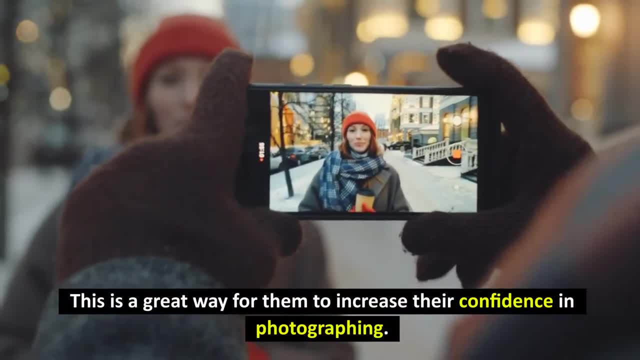 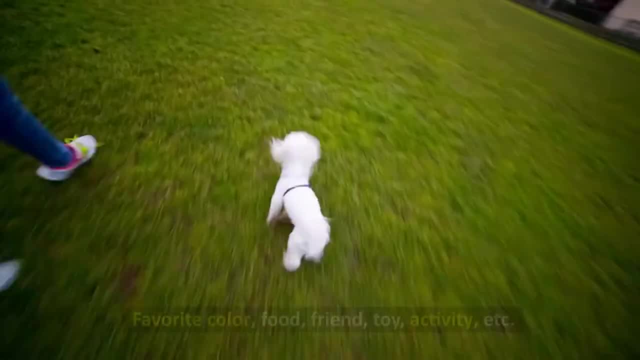 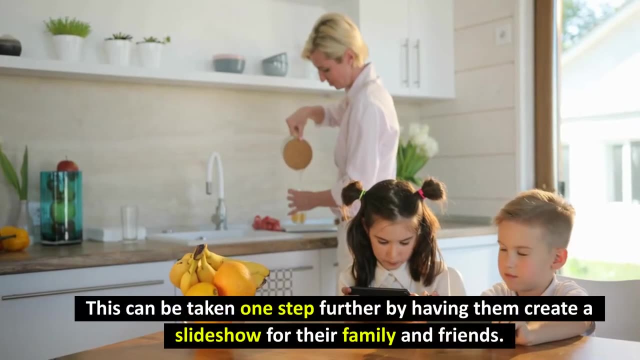 and then print it out again. This is a great way for them to increase their confidence in photographing My favorite things. Ask your child to take five photos of their favorite things: Favorite color, food, friend toy, activity, etc. This can be taken one step further by having them. 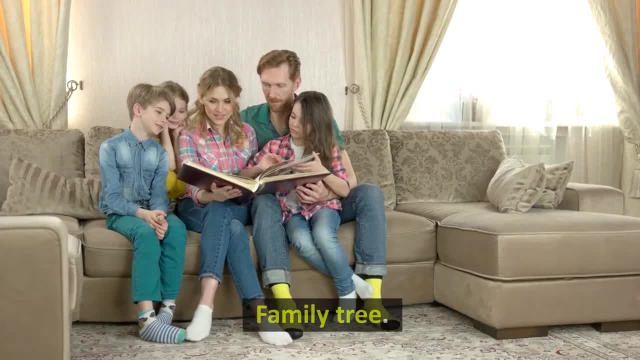 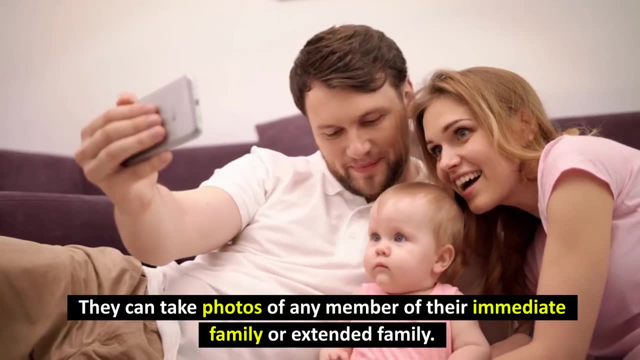 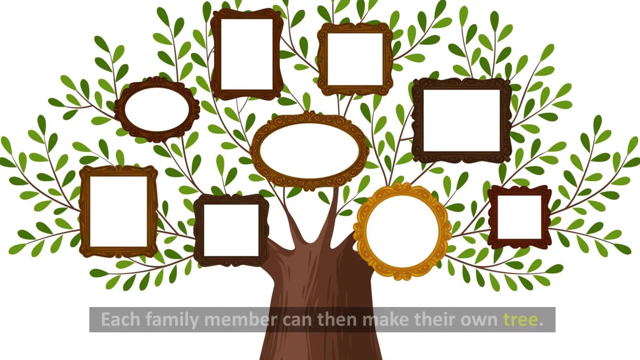 create a slideshow for their family and friends Family tree. Ask your child to take portraits of their family. Don't forget about the pets. They can take photos of any member of their immediate extended family. Next, create a tree, either on paper or on the computer. Each family member can. 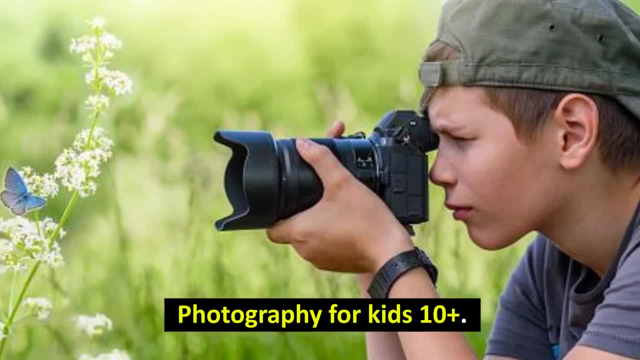 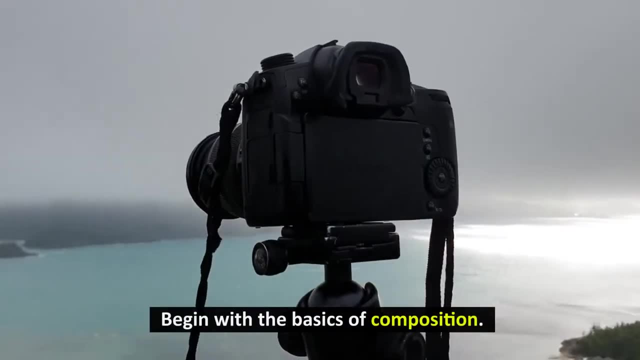 then make their own tree Photography. for kids 10 plus, Begin with the composition. This age group can learn even more about photography. Begin with the basics of composition. Your child will be able to tell a better story by teaching them how to add variety and composition to their photos. 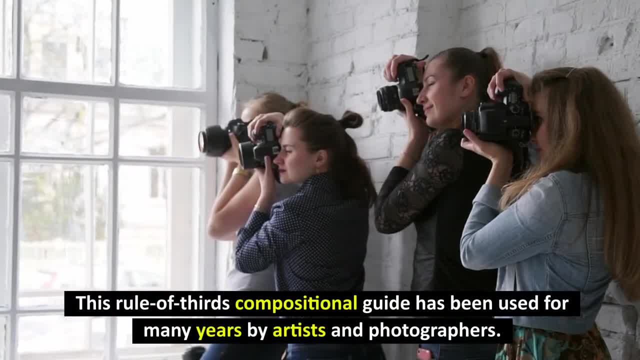 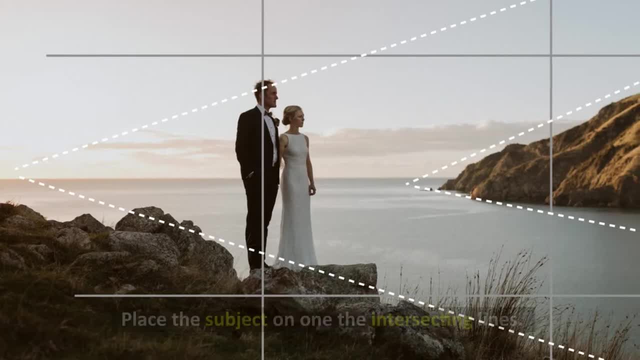 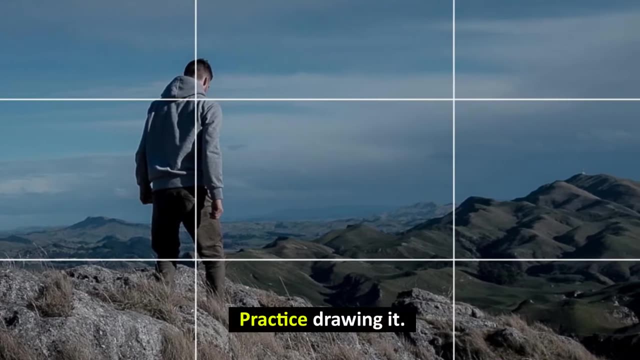 Rule of thirds. This rule of thirds compositional guide has been used for many years by artists and photographers. Allow them to view the scene as if it were a tic-tac-toe board. Place the subject on one the intersecting lines To help them visualize it. draw it on another photo. Practice drawing it. 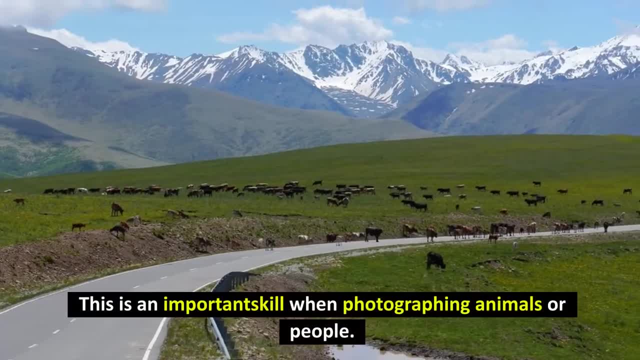 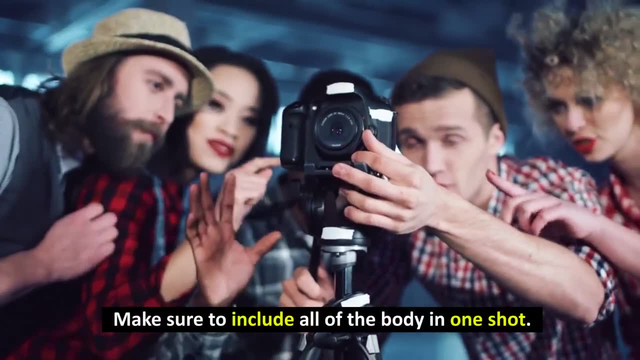 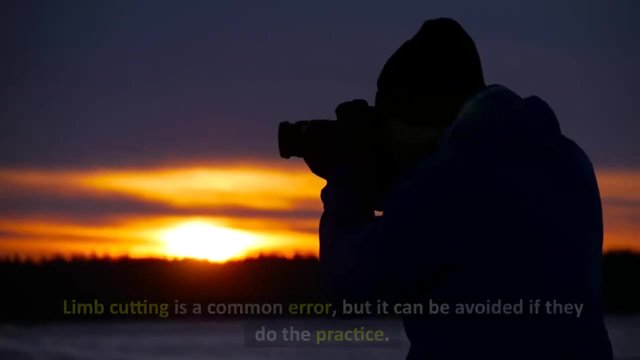 Limb chops. This is an important skill when photographing animals or people. If the joint bends, you should not crop your subject. Make sure to include all of the body in one shot. Once they are done, ask the child to show you each joint. Remind them not to crop the subject. Limb cutting. 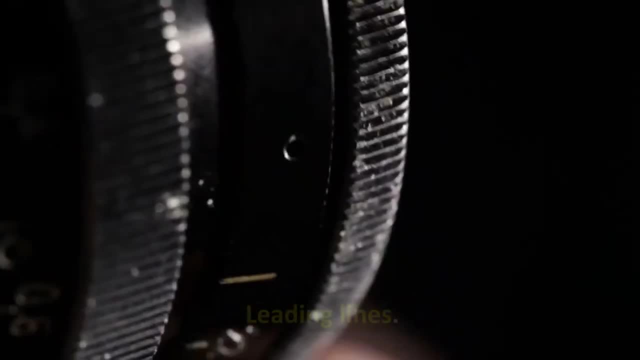 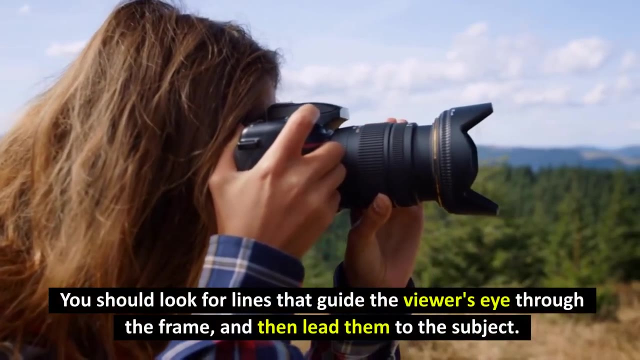 is a common error, but it can be avoided if they do the practice Leading lines. This is a favorite technique of mine and an advanced one. You should look for lines that guide the viewer's eye through the frame and then lead them to the subject. Lines will be found on sidewalks and on buildings, Even. 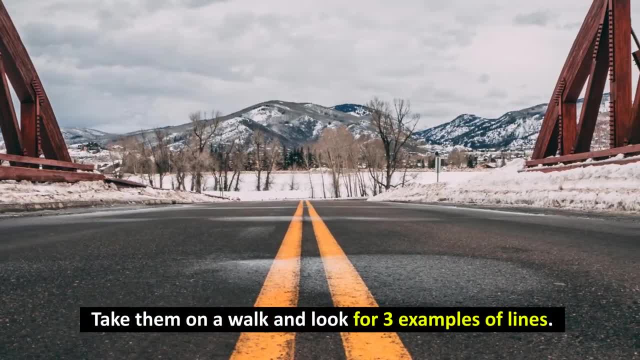 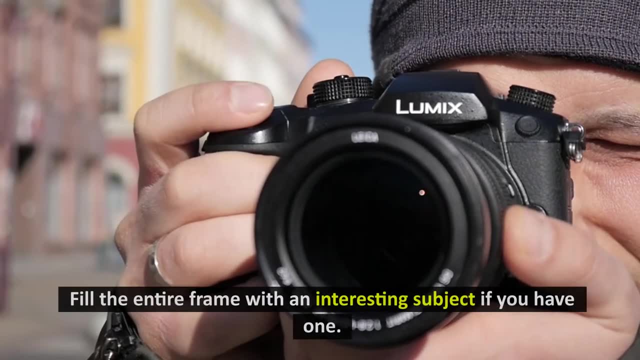 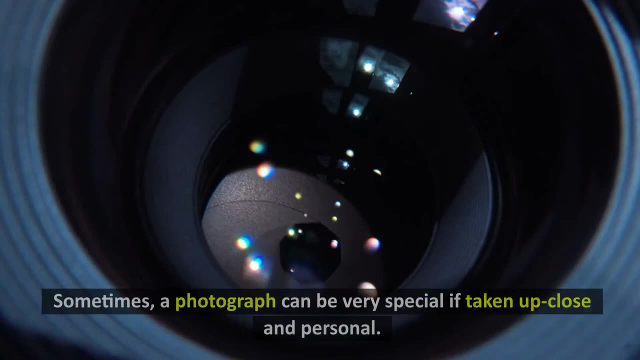 an arm can lead to a line. Take them on a walk and look for three examples of lines. Ask them to take photos of the leading lines. Fill the frame, Fill the entire frame with an interesting subject. if you have a lot of time, Photograph a bicycle wheel, a flower or fun pattern. Sometimes a photograph can. 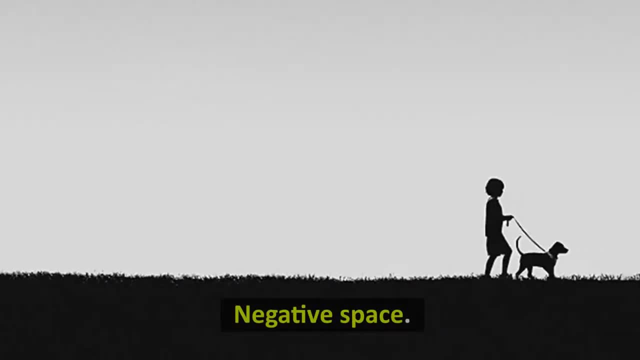 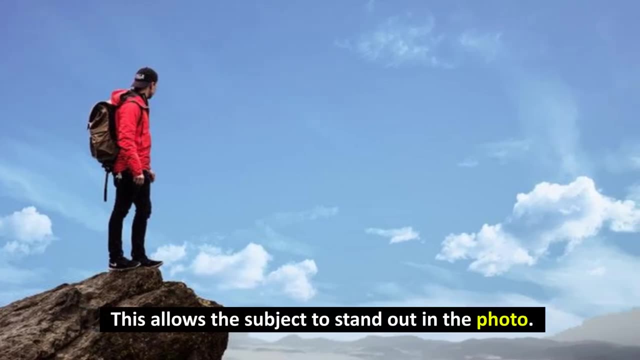 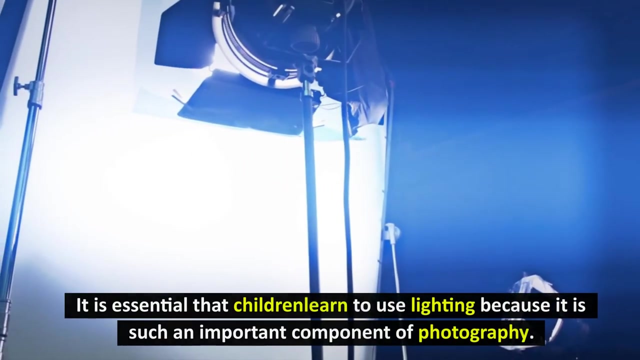 be very special if taken up close and personal. Negative space: A powerful composition technique is to use negative spaces. This allows the subject to stand out in the photo. This can give the subject a dramatic look that will really make it pop. Lighting can also be tackled. It is essential. 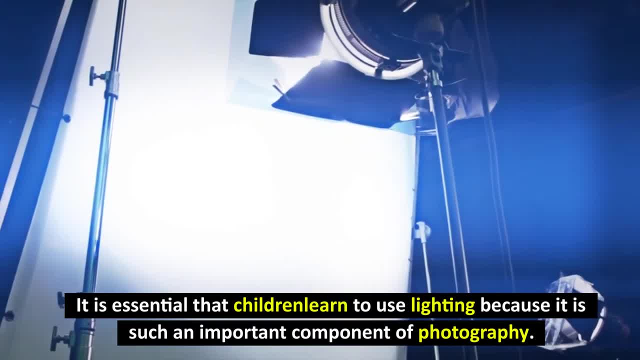 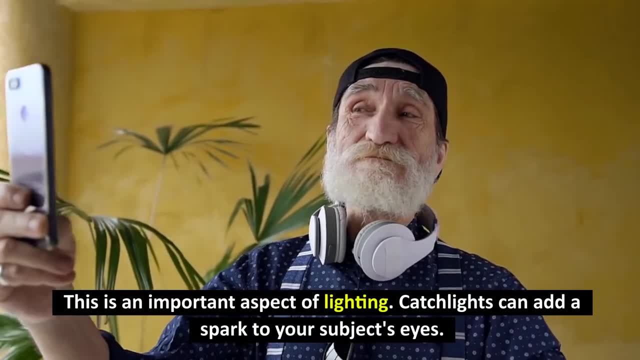 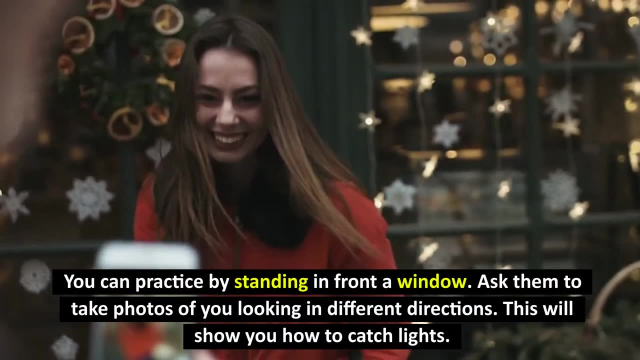 that children learn to use lighting because it is such an important component of photography. Catch lights. This is an important aspect of lighting. Catch lights can add a spark to your subject's eyes. You can practice by standing in front of window. Ask them to take photos of you looking in different directions. This will show. 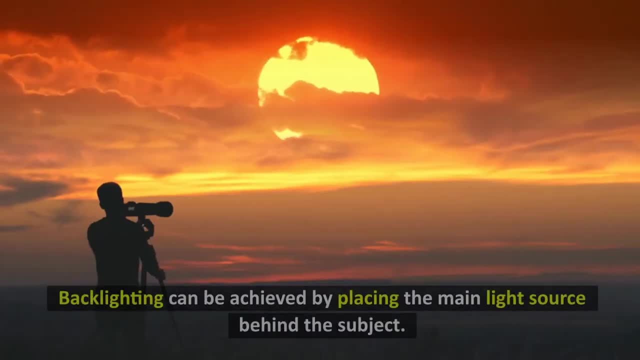 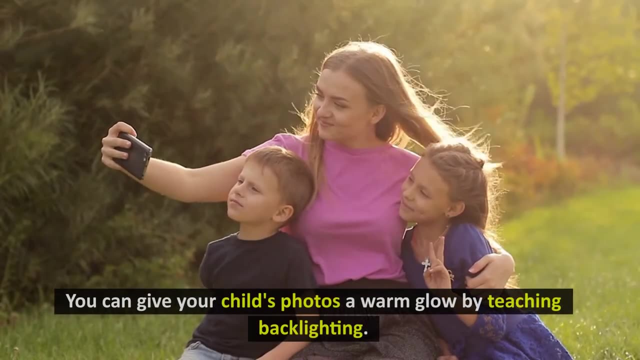 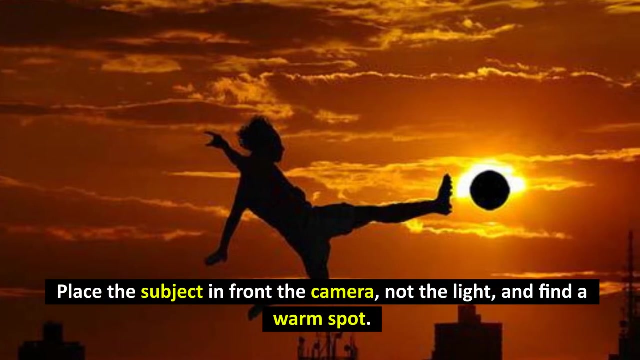 you how to catch lights Backlighting. Backlighting can be achieved by placing the main light source behind the subject. This effect is best at sunset. You can give your child's photos a warm glow by teaching backlighting. Take a walk about an hour before sunset. Place the subject in front. the 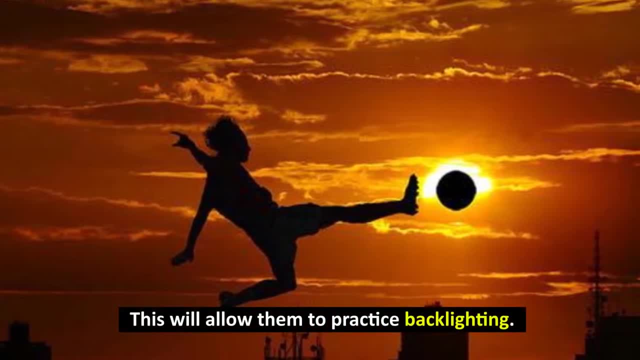 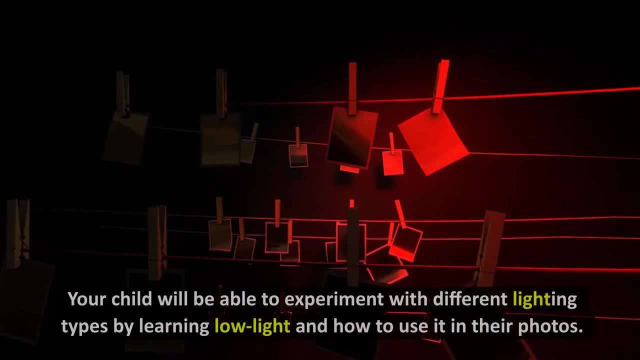 camera, not the light, and find a warm spot. You can also take photos of your child in front of a light source. This will allow them to practice backlighting, Low light- Sometimes we live in rooms with very little natural light. Your child will be able to experiment with different lighting. 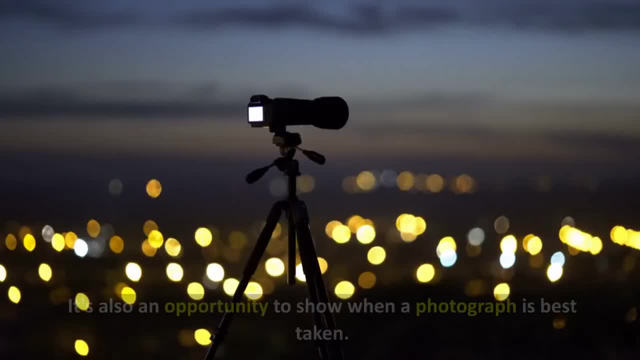 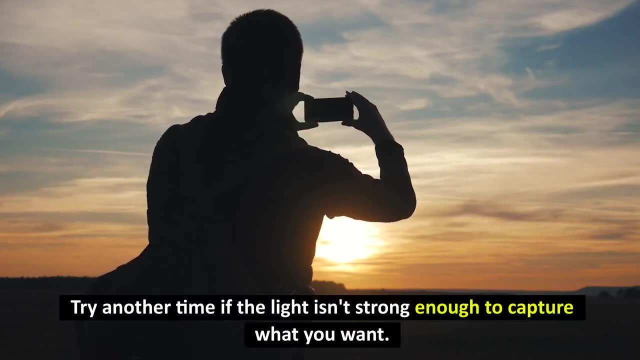 types by learning low light and how to use it in their photos. It's also an opportunity to show when a photograph is best taken. Try another time if the light isn't strong enough to capture what you want. Window light: This is the most common type of natural lighting, Sometimes window lights. 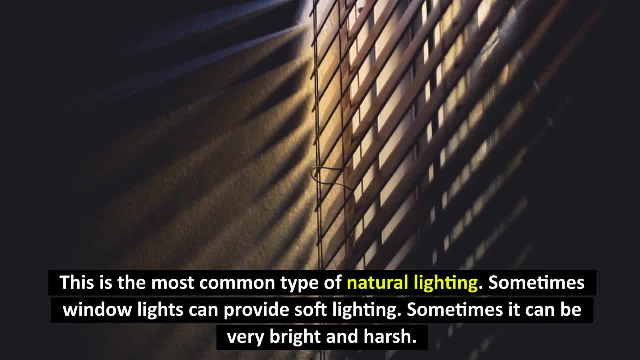 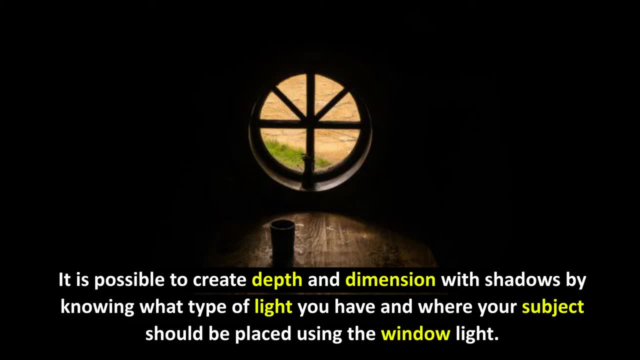 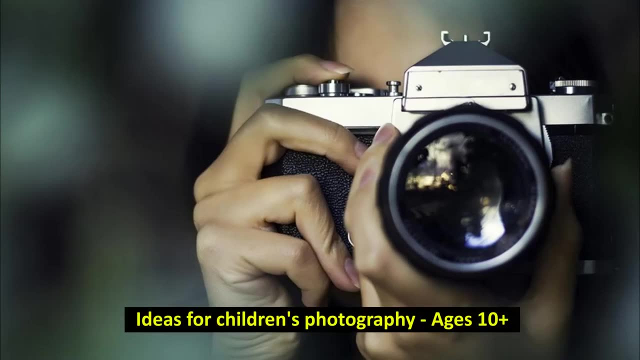 can provide soft lighting. Sometimes it can be very bright. It is possible to create depth and dimension with shadows by knowing what type of light you have and where your subject should be placed. using the window light For dramatic lighting create big shadows in your photograph. Ideas for children's photography: Ages 10 plus. Skill building: You can. 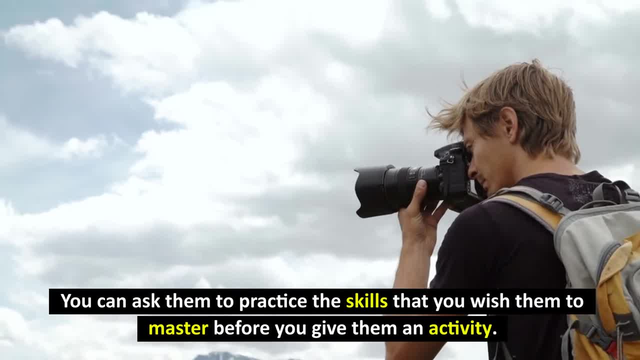 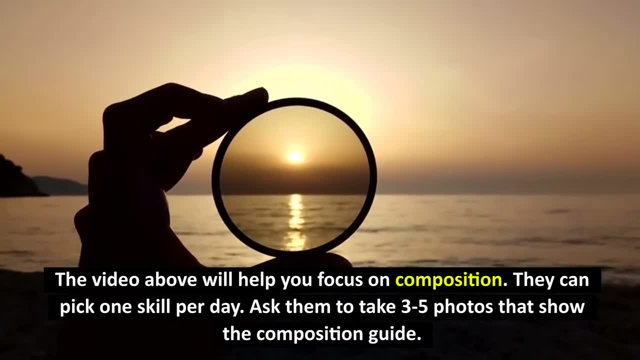 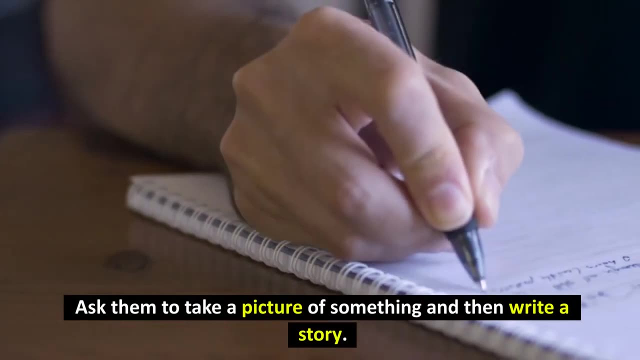 ask them to practice the skills that you wish them to master before you give them an activity. The video above will help you focus on composition. They can pick one skill per day. Ask them to take three to five photos that show the composition, A story guide, story time. ask them to take a picture of something and then write a story. 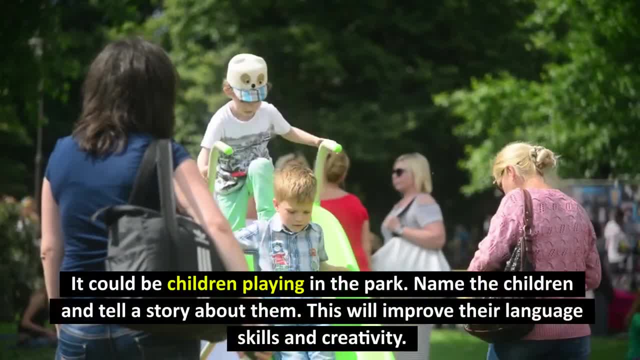 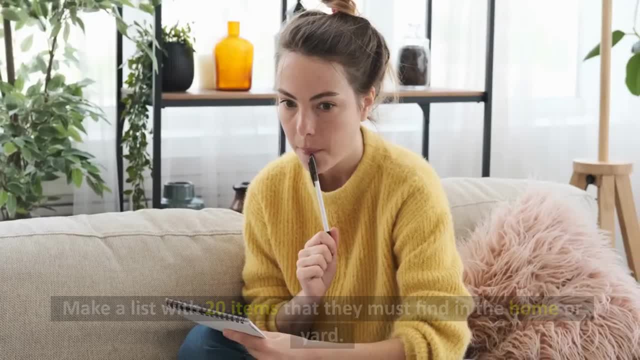 it could be Children playing in the park. name the children and tell a story about them. this will improve their language skills and creativity. scavenger hunt: make a list with 20 items that they must find in the home or Yard. give them the camera and let them take photos of the possibilities. 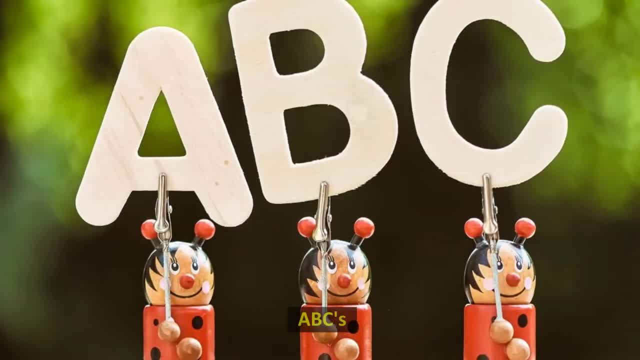 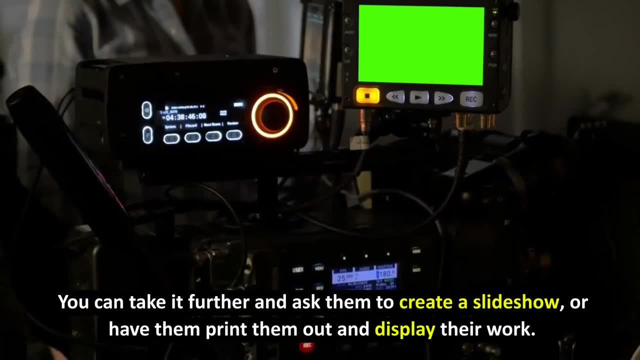 you should always be up for a challenge. ABCs ask them to take a photograph of something that begins with each letter in the Alpha. You can take it further and ask them to create a slideshow or have them print them out and display their work. 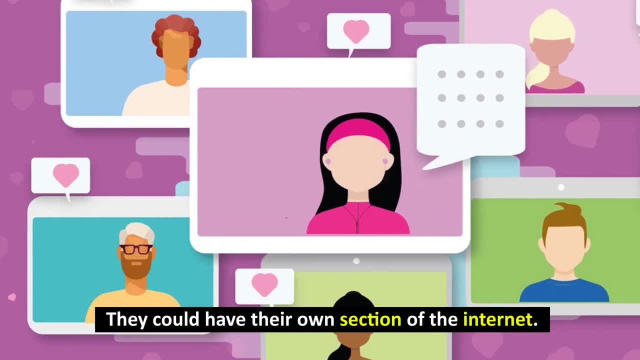 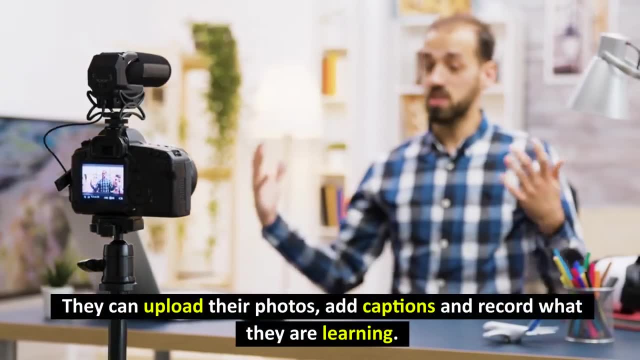 Create your blog. They could have their own section of the internet. If you wish, you can make their blog private so that only your family can view it. They can upload their photos, add captions and record what they are learning. You can take their photos and tell them stories and put them together in a digital album. 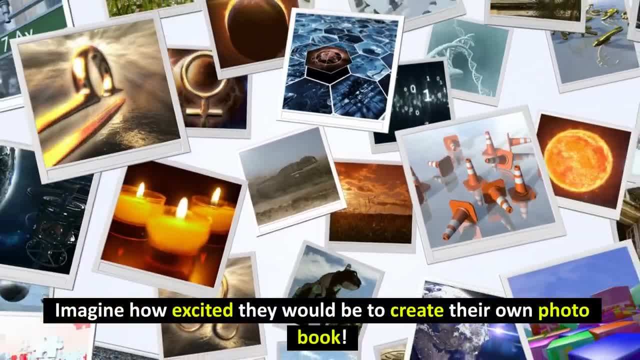 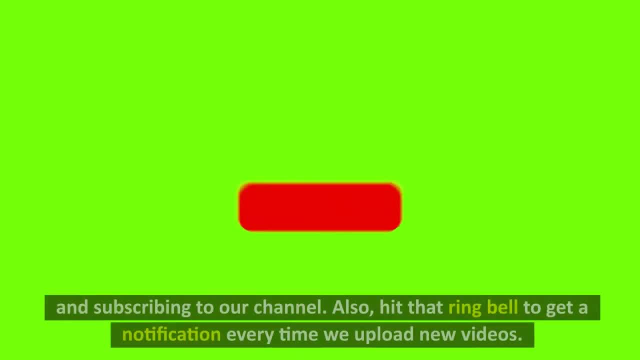 Imagine how excited they would be to create their own photo book. Thank you for watching. If you like the video, please support our channel by liking this video And subscribing to our channel. Also, hit that ring bell to get a notification every time we upload new videos.